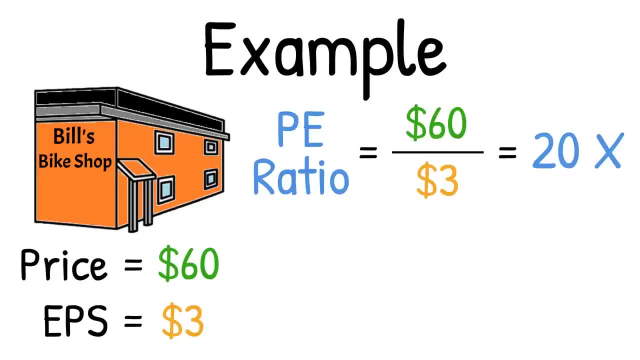 is currently valuing the shares of Bill's Bike Shop at 20 times the amount of their yearly profit. So if you were to buy shares in Bill's Bike Shop, you would be paying 20 times the amount that they generate in profit for the year. This ratio also implies that it would take 20 years. at current 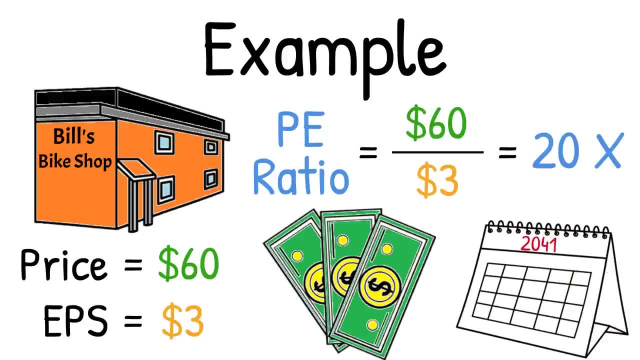 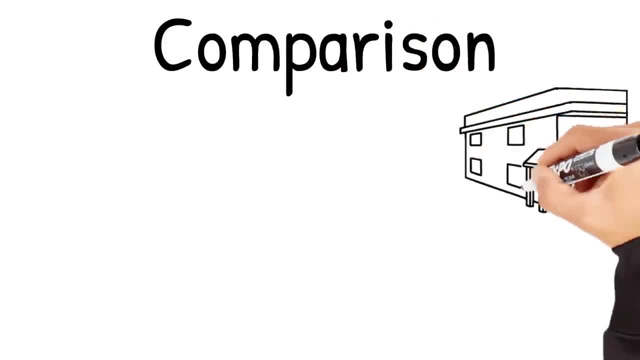 price and profit levels for Bill's Bike Shop to make enough money to pay back all the shareholders in full for their shares. P-E ratio really shows its strength when you use it to compare different companies within the same industry to get a better idea of how each company is being valued. 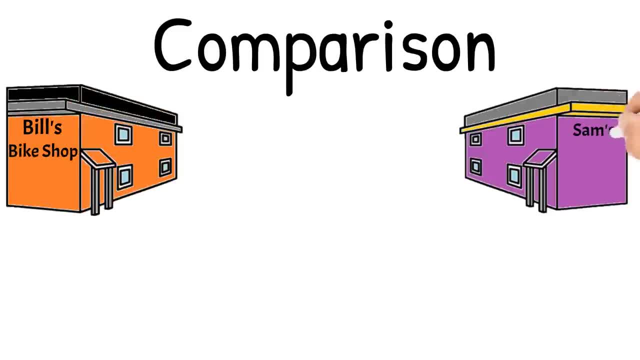 Let's compare two companies here: Bill's Bike Shop and Sam's Scooter Company, Both of which provide alternative means to transportation, so we can consider them to be in the same industry. From before we already know that Bill's Company has a price per share. 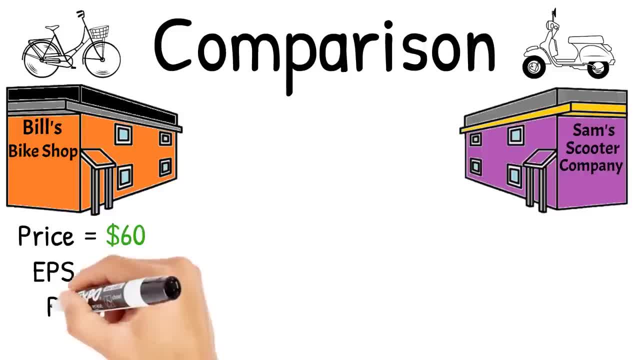 of $60 and an earnings per share of $3, giving us a P-E ratio of 20 times. Now for Sam's Scooter Company, they currently have a price per share of $75 with an earnings per share of $5.. You may be. 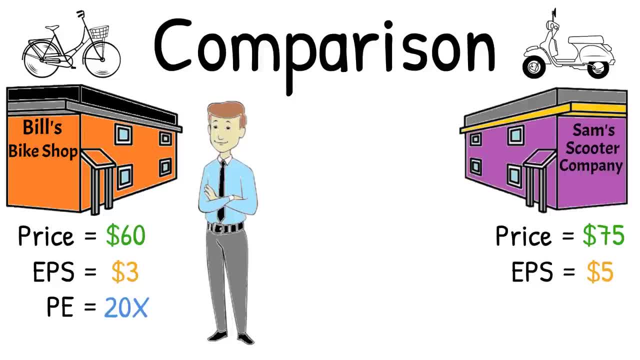 inclined to think that Bill's Bike Shop is a better value because the share price is only $60 versus the $75 for Sam's Scooter Company. But if you were to buy shares in Bill's Bike Shop, Sam's Scooter Company has a P-E ratio of 15 times. So what's going on here? Even though Sam's 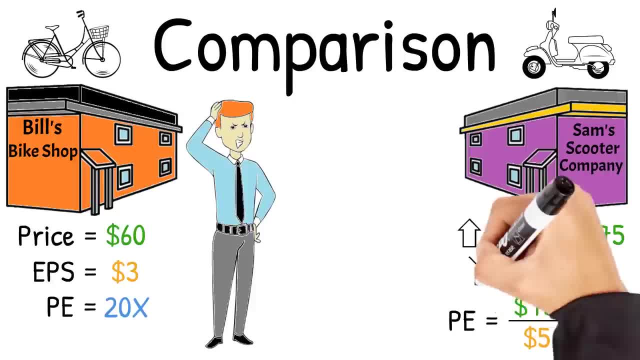 Scooter Company has a higher price per share. they are also generating more earnings for the shares outstanding. What we see is that when we compare the two companies, and in apples to apples sense, with P-E ratio, we find that Sam's shares are actually of better value, since the company 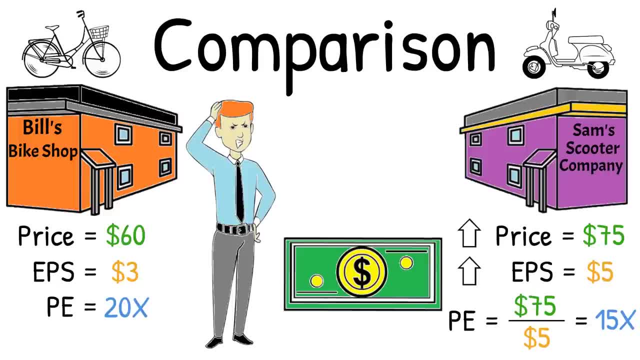 is more profitable. Even though Sam's Scooter Company shares are higher, they are also generating more profits than Bill's Bike Shop. You have the right to $5 per share with a profit, instead of only the $3 per share in profit that Bill's Bike Shop offers. This is really the key to understanding. 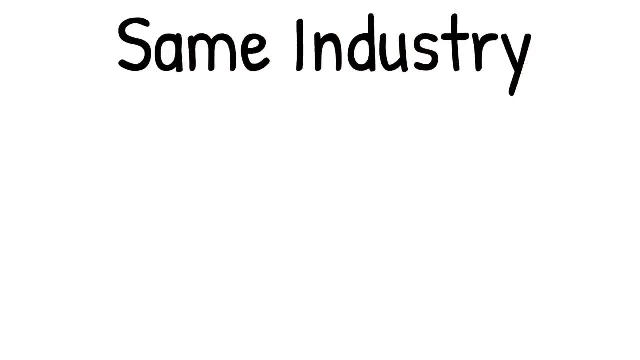 what P-E ratio tells us. You should know that the price to earnings ratio is really only useful when comparing companies within the same industry, as different industries will have different standards when it comes to P-E ratio. It would not make sense to compare McDonald's P-E ratio.